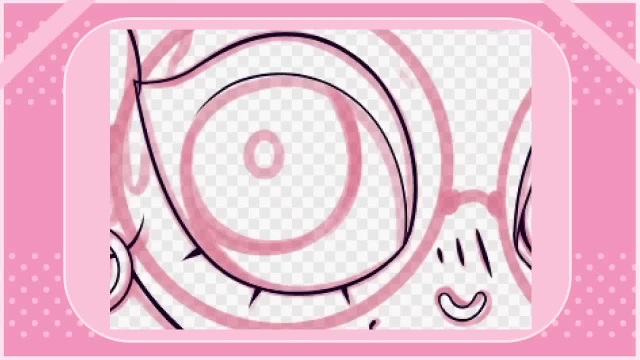 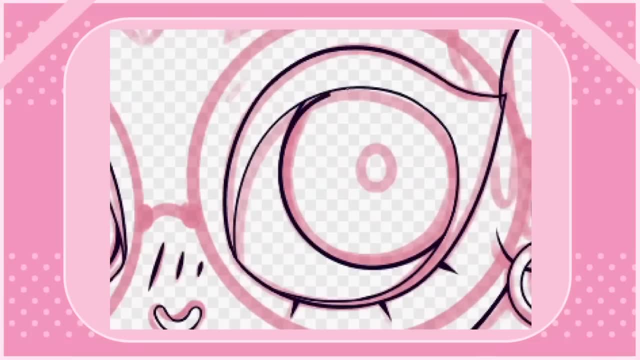 cuphead artwork still in my DeviantArt- and I was only paid a total of ten dollars for all three. Outside of that, I made a lot of art for friends, all for free, and in retrospect I do think that a lot of people became my friend, especially in middle school, just to get free art out of me. 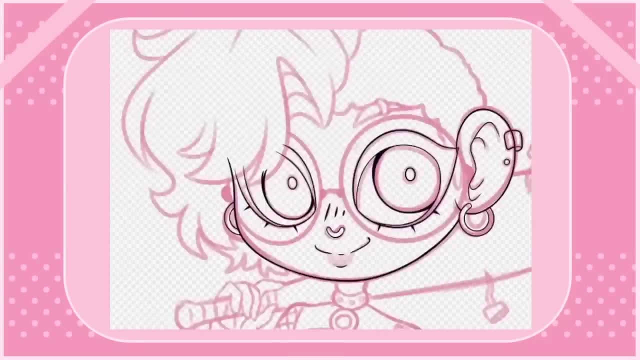 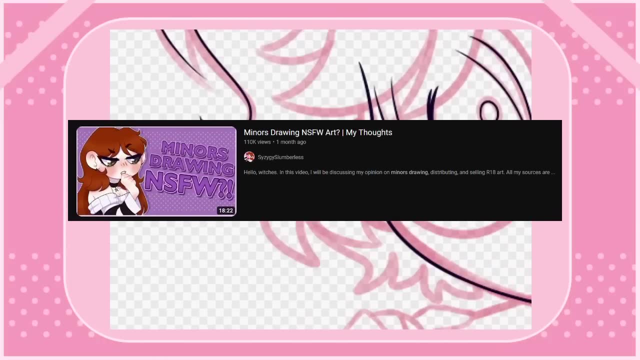 Not all, of course, but many. This actually happened online a lot as well, but actually not with friends. I revealed a previous experience in my Miner's Drawing Not Safe for Work video, in which a guy in his thirties asked me, a fourteen-year-old to draw him not-safe-for-work of an anime girl he liked. 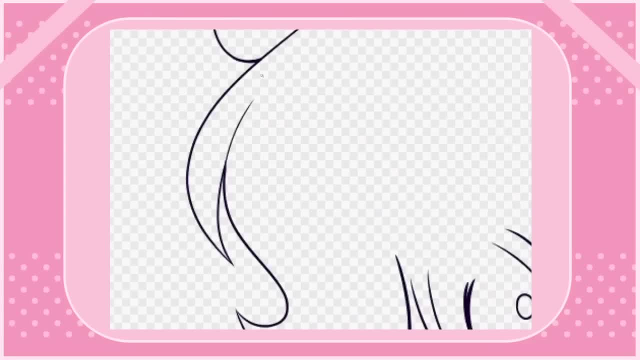 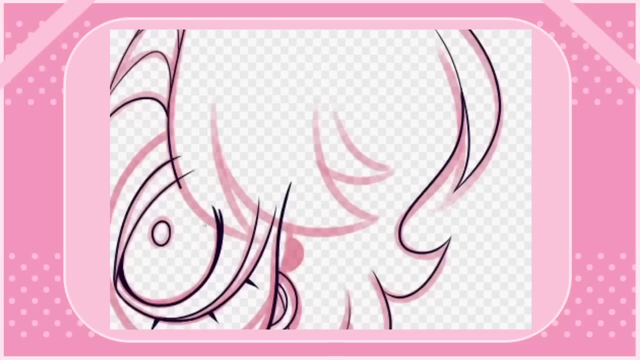 At the time, I didn't really see value in my work and I just did what he asked. Even outside of this particularly creepy experience, I remember like two other occasions in which I was requested art and I just did it without payment. This is a big no-no, guys. Of course it is up to you as the artist. 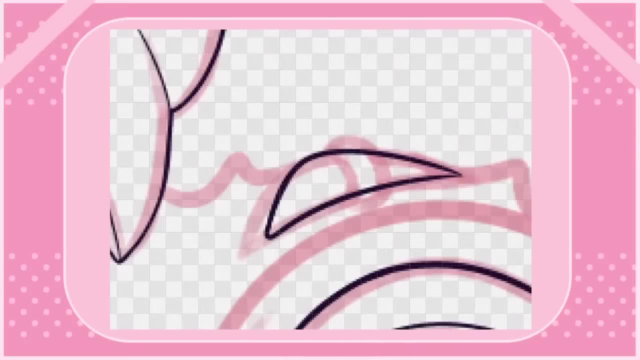 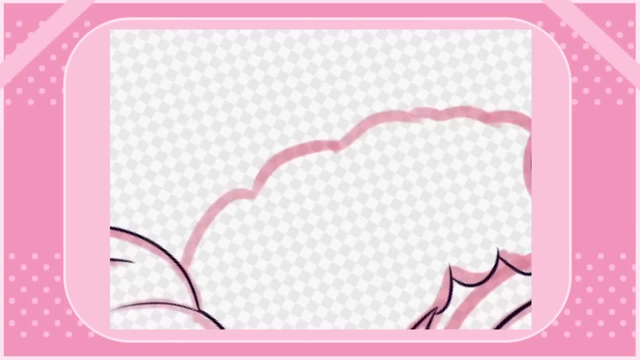 to decide whether or not you charge friends for your work, but if the reason that you're giving artwork out for free is because you think that your work is not worth being paid for, then I'm here to say that you're wrong. But like in the nicest way possible, of course. 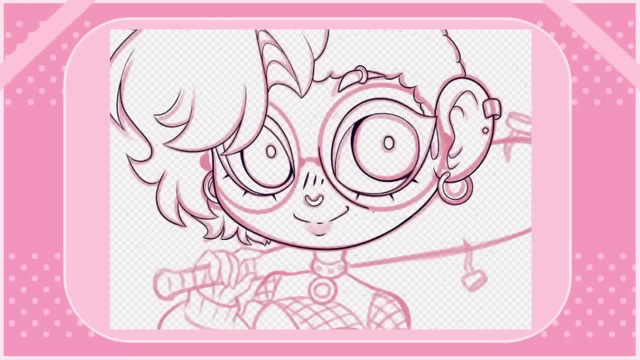 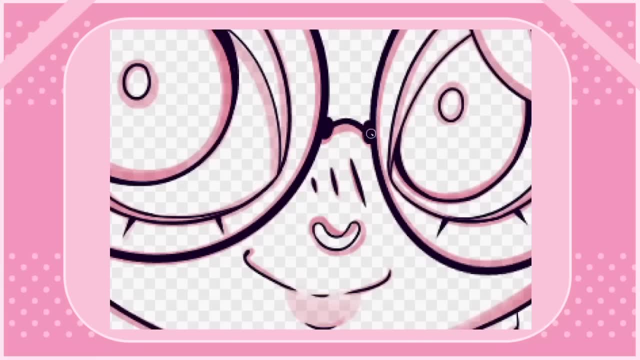 Your time and work is worth being paid for. so when you set the price of your commissions, don't be afraid to charge a decent amount. If people want art from you, then they can pay you for your time and your skill. Art is not an essential good. 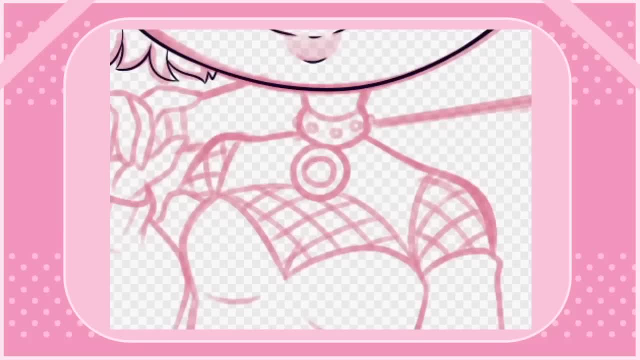 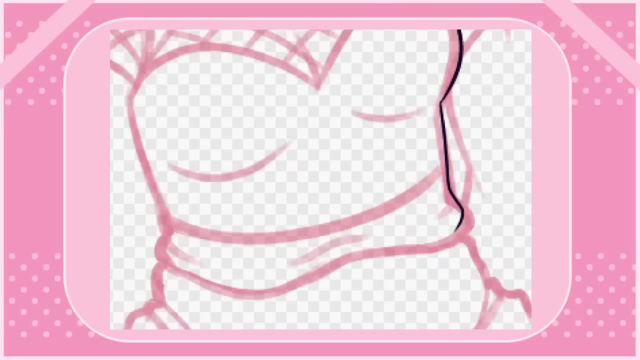 it's rather a luxury and no one is owed anything from you without any payment. Another thing that I think that is important for young artists to know is that when you first open commissions, you aren't gonna get very many of them, Especially if you have a smaller viewer base and subscriber or follower count. 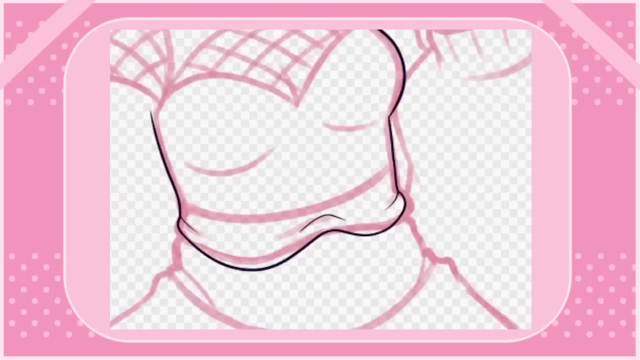 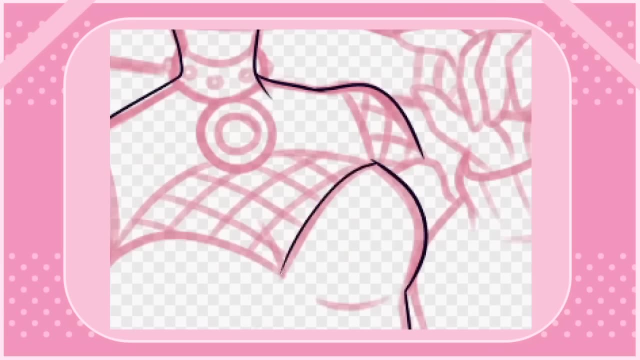 it may take a while for you to get your first commission. I had commissions open for actually like quite a few years and then, when I was a YouTuber, quite a few months before I ever got commissioned, and for insanely low prices as well. 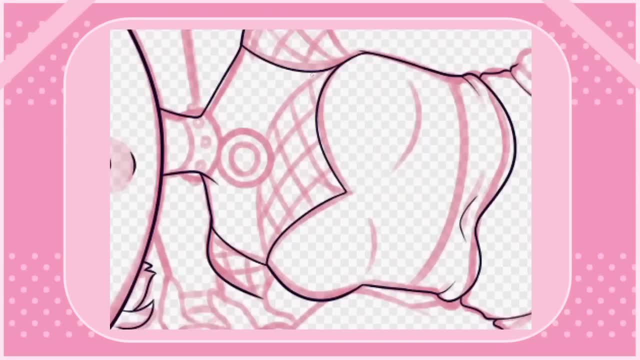 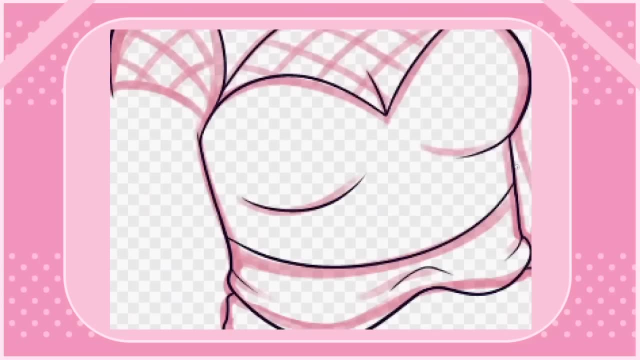 So if you don't get any offers right away, don't get discouraged. It doesn't mean that your work isn't good, but it may mean that you need to promote yourself more and build more of an audience and a portfolio. Another thing that every artist needs to know is that you have the right to deny. 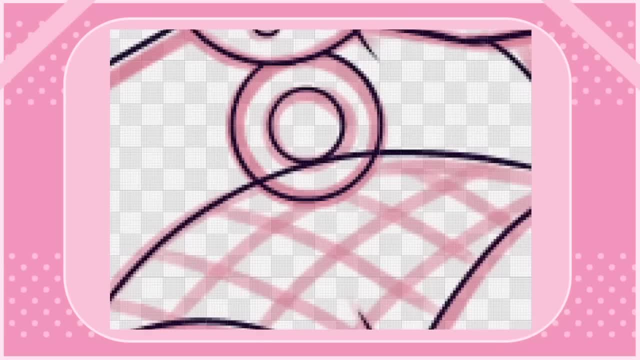 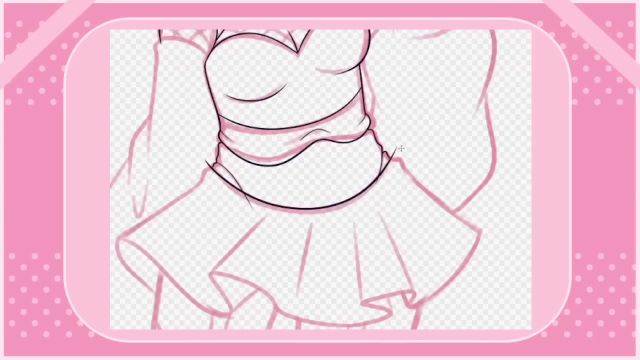 any commission or request that comes your way. If you're too young or uncomfortable with drawing suggestive not-safe-for-work or gore art, you can turn down that commission. And if you don't know how to draw something that they're asking for. 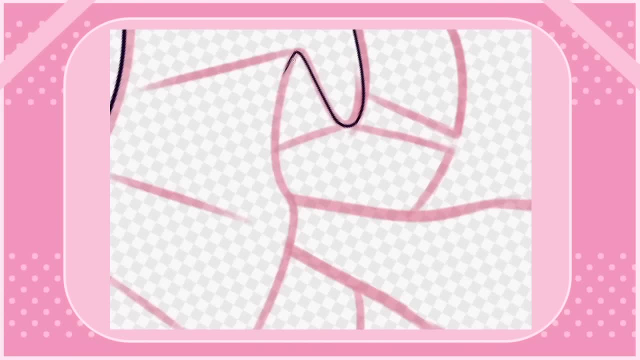 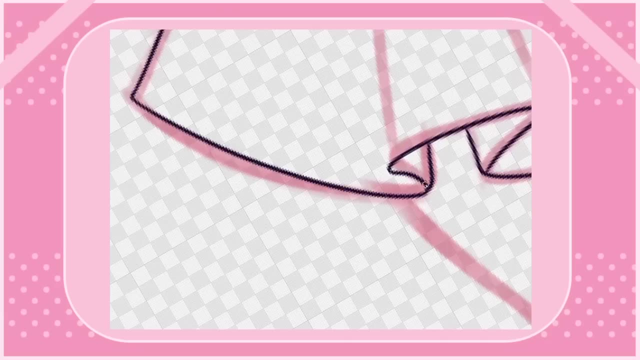 feel free to direct them elsewhere. Even if you make a post asking for requests or art ideas, you can still deny each and every one if they don't suit your interests or taste. Again, no one is entitled to your work and it's important that you stick within your comfort zone and put your foot down when you need to. 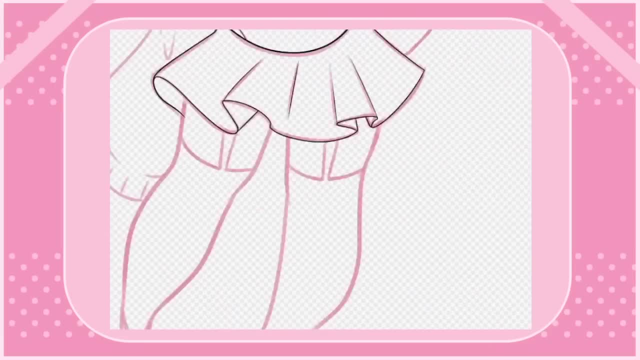 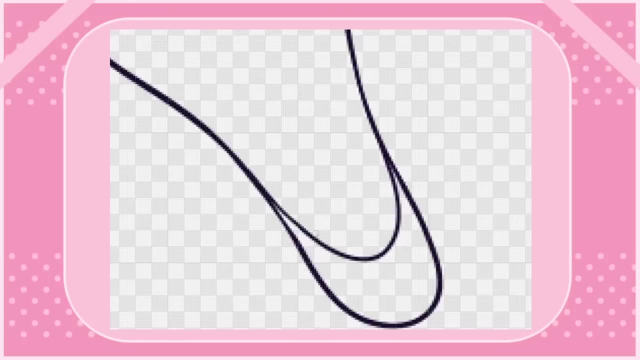 Trust me, I know the ramifications of not doing so from experience. it may seem hard to assert yourself at first, especially when it comes to someone offering to pay you, but I assure you that it will save you a lot of grief in the long run. 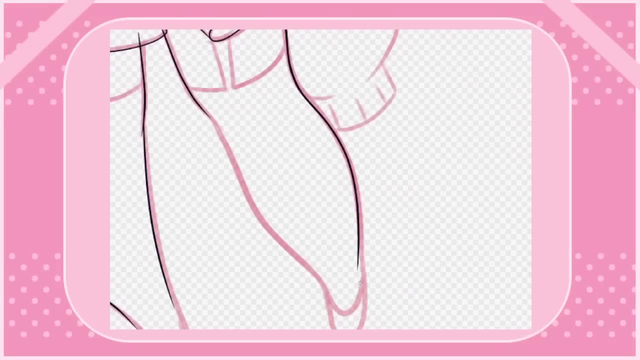 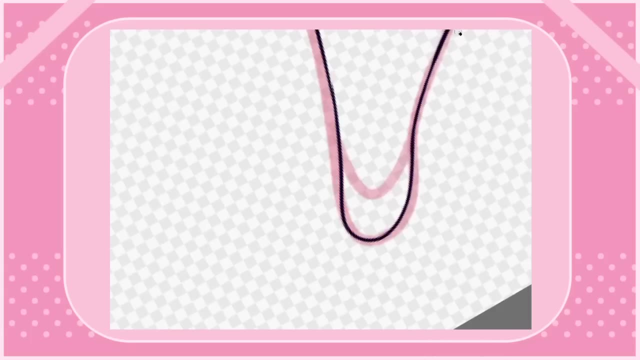 Next up: use references, And I know that may seem like a very basic tip, but let me tell you it's definitely an important one that you should always remember. When I was younger, I rarely ever used references and rarely ever even traced. 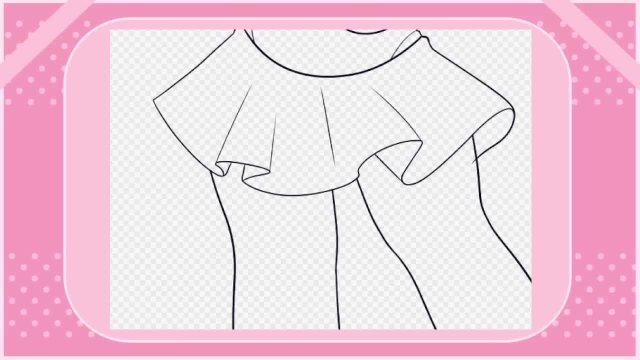 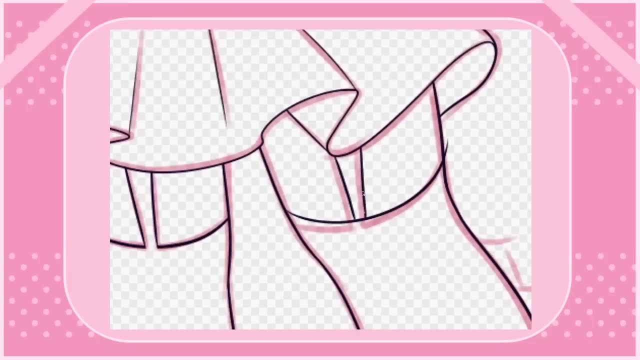 so it was difficult for me to learn proper anatomy and posing for a while earlier in my art career. I still use references when it comes to almost any drawing that I do, especially when it comes to more complicated posing and piece composition. Also remember to use a variety of references. 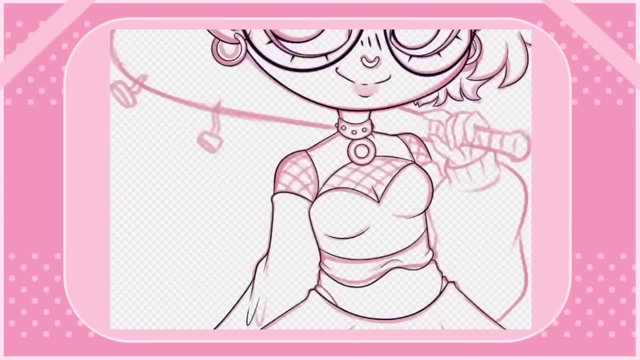 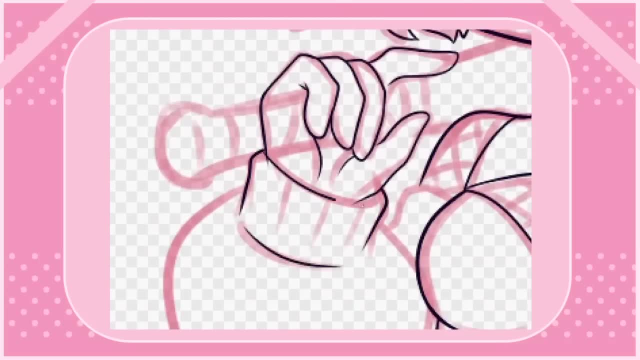 When I was first starting out, I either never used references at all or the ones that I did use were all in the anime style and were sourced from a couple how-to-draw books that I had as a kid, or from really spindly art style like Vivzie Pops and Twisted Doctors. 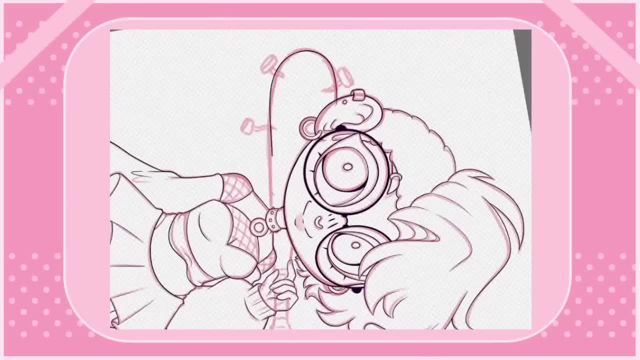 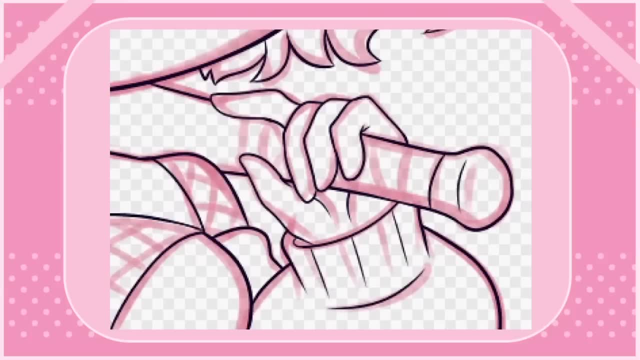 This meant that I would often copy anatomy mistakes that were present within those inspirations. Because I was so often overexposed to skinny characters, I tended to draw limbs that were too thin. I tended to draw limbs that were too thin. I tended to draw limbs that were too skinny for my art style. 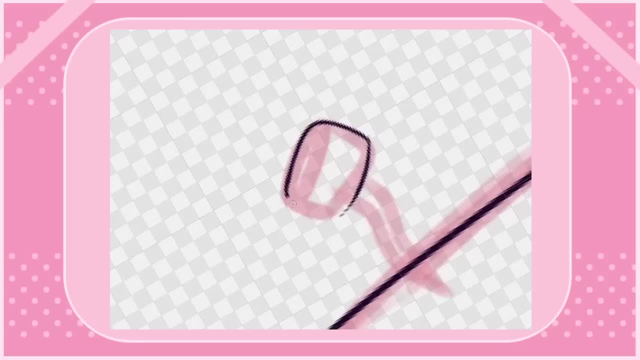 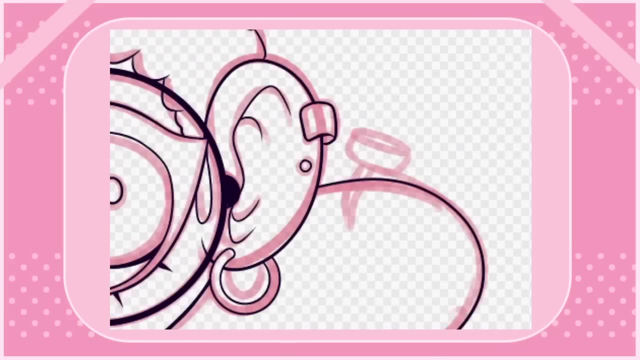 and it took a while for me to unlearn and correct a lot of those tendencies. Sometimes I even struggle with it to this day. So in that case I would recommend making inspiration and anatomy folders full of references for your art and try to take them from a lot of different sources so that you have a fuller scope of things. 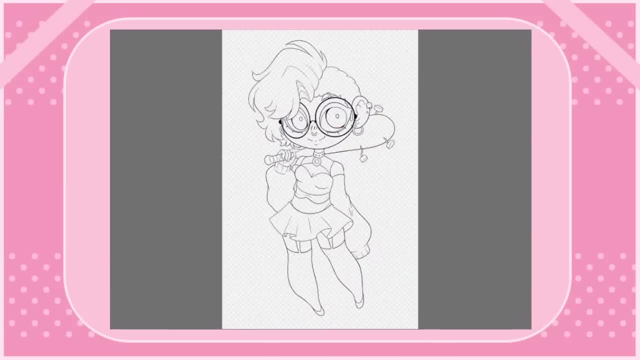 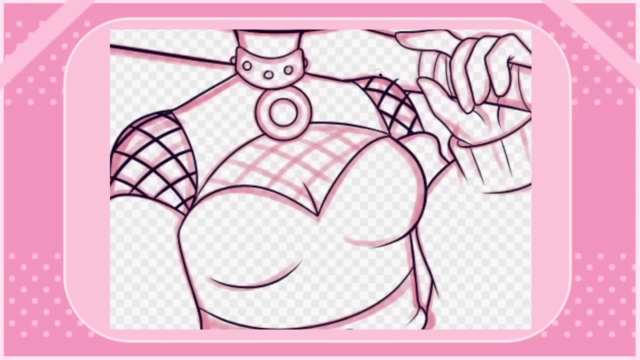 Especially if you have an art style that is closer to realism. when it comes to anatomy, I also recommend referencing real photographs, and if you have a mirror or a good place to prop up your phone, you can even take pictures of yourself to reference your own anatomy and poses. 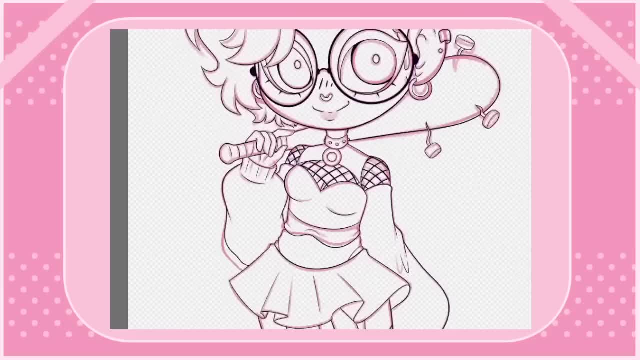 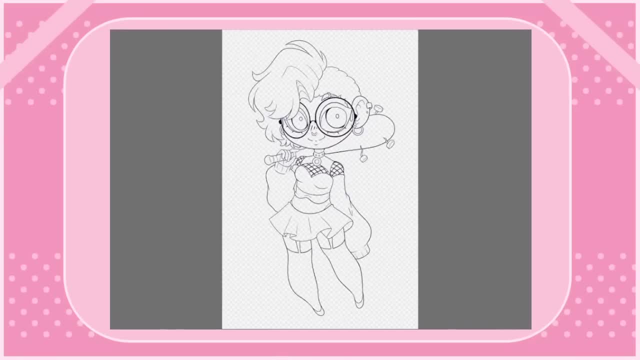 Another tip that kind of goes along with the reference thing that I also recommend is that you try drawing in different styles and experiment. You don't need to pick one and just stick to it for the rest of your life. You can move out of your comfort zone and try new things as well. 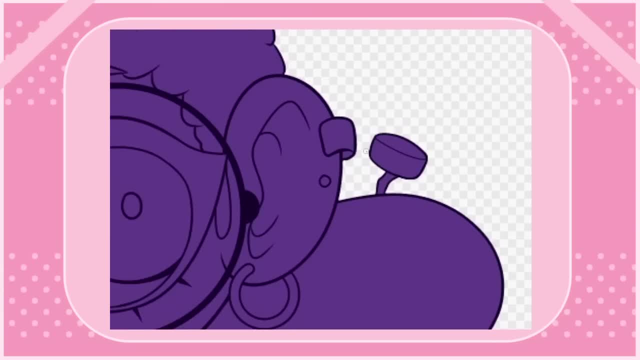 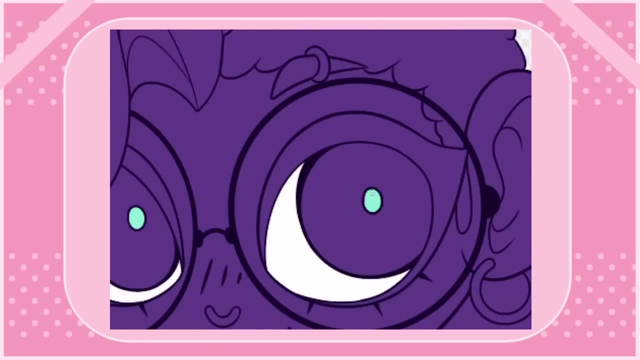 Don't get too into your head trying to develop your art style. It will develop on its own Experiment. draw the things that you want to draw and that you think look good, and you'll find what you're passionate about. Next up, here's one tip that I'm unfortunately super guilty of. 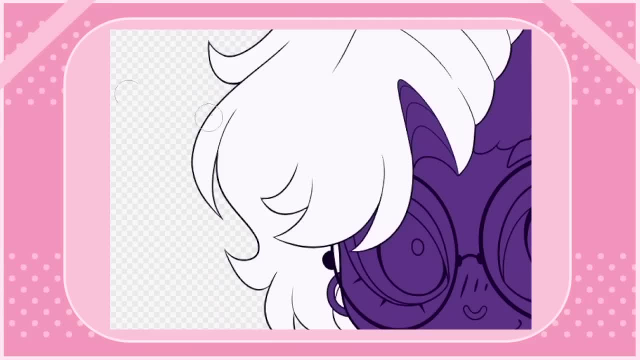 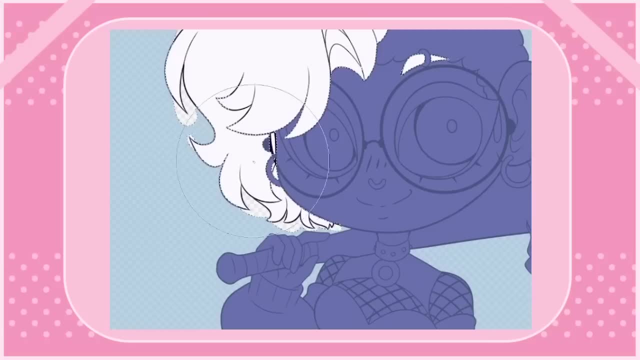 Even to this day I sort of struggle with it. Not everything you draw has to be a grandiose, fully rendered, perfectly drawn and lined detailed piece. I've noticed that doodling occasionally has actually helped me progress in my art. 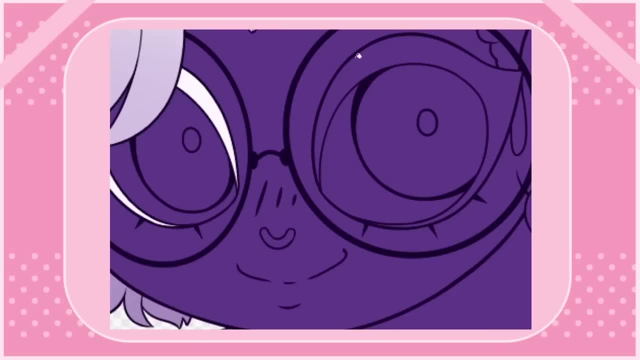 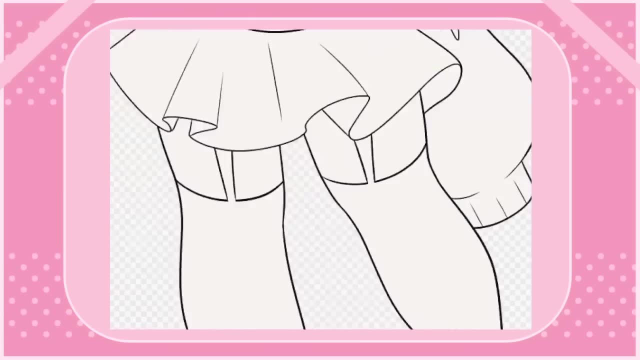 and, to be honest, I should probably doodle more often. even to this day, I tend to kind of get in my head about my art, thinking that everything has to be fully shaded and rendered and detailed, Especially if you're a new artist that struggles doing all of that. 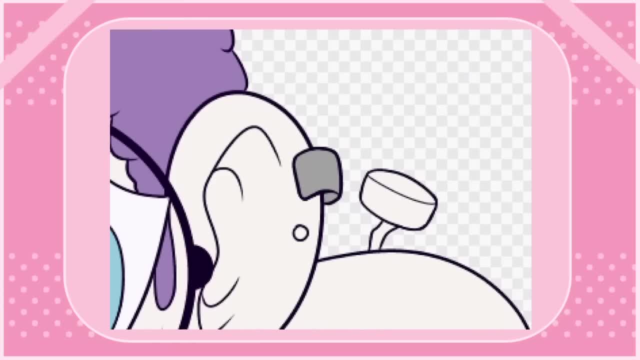 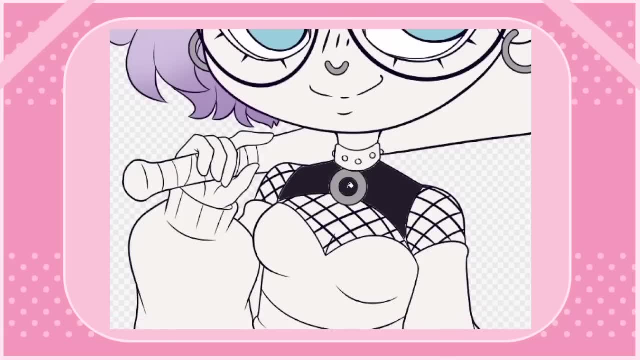 I would see how not taking the time to practice doodle and have fun could actually stunt growth. So I would recommend taking a more lax approach to working on your skills. Of course, that doesn't mean you should never put your effort into drawing those fully rendered. 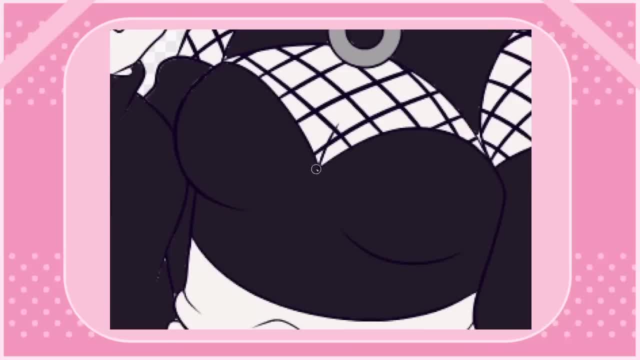 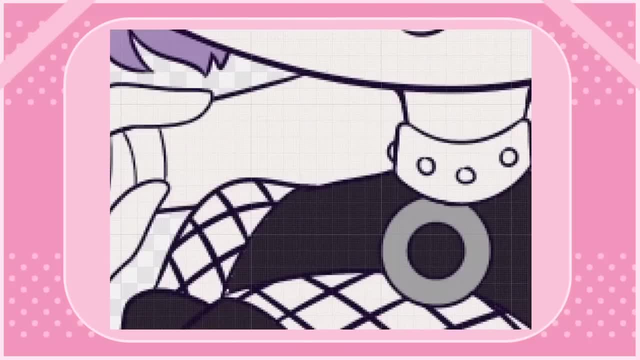 pieces, but just know that you can practice in other ways too and have fun while doing it. Another tip that I have is to not get too in your head about your own improvement and to never compare your worth to that of another artist. 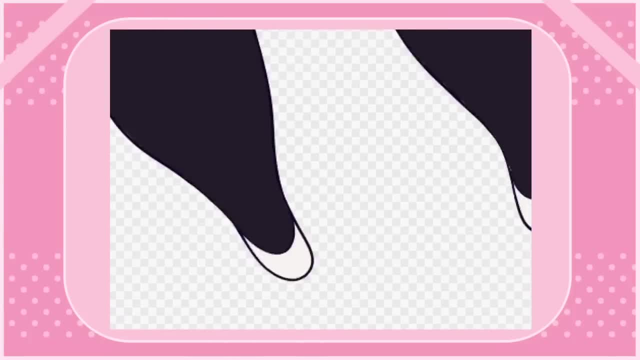 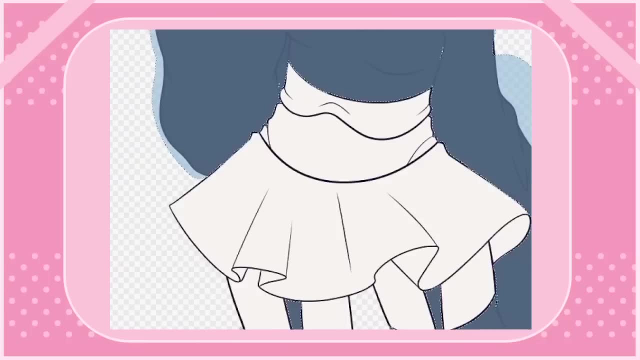 I know from experience that being an intermediate artist is extremely difficult. When you first start in art you'll see a lot of rapid improvement as you learn the basics and develop your style. But once you get to a certain point of development the improvement will start slow and visible improvement will be less easy to take notice. 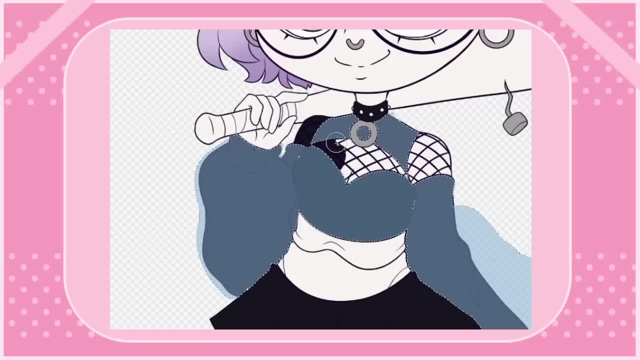 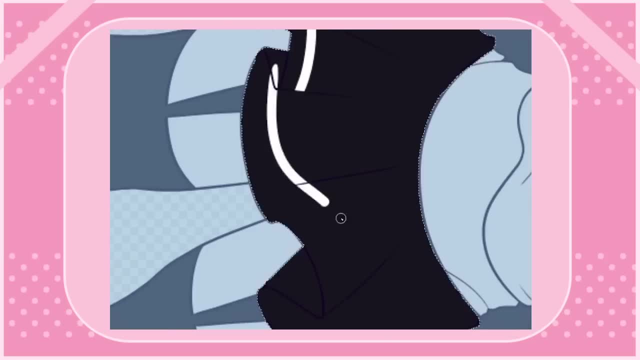 of. Of course. that doesn't mean that you've stopped improving- definitely not. It just doesn't come as fast as it may have before. When you're in a rut like this, don't compare yourself to other artists, Don't dog on yourself or get down on yourself because you think that their work is better. 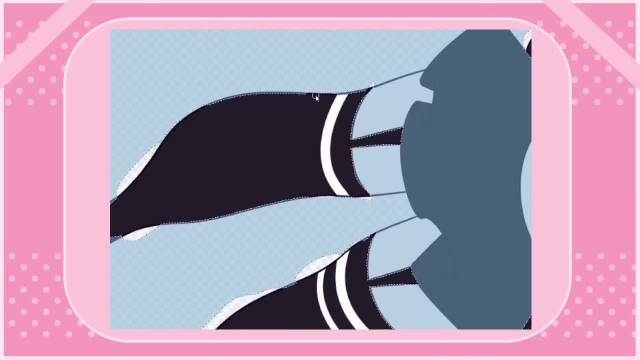 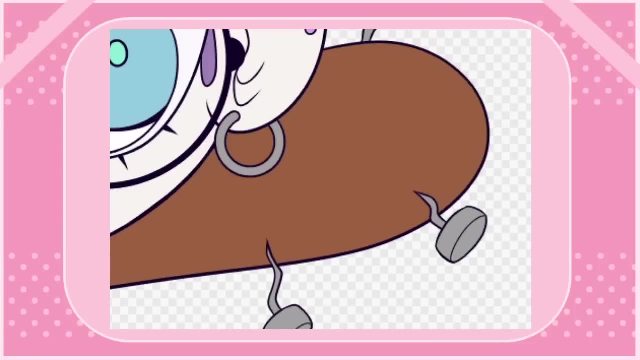 or because they have more of a social media presence or because they get more commissions than you. None of that indicates that you're worthless in comparison. Self-deprecating really doesn't lend well to improvement, and it may make you start to slowly hate yourself. 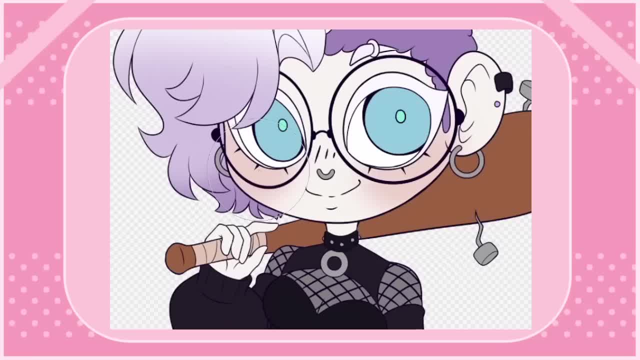 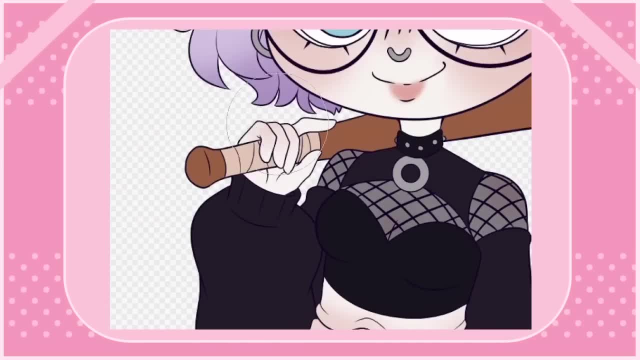 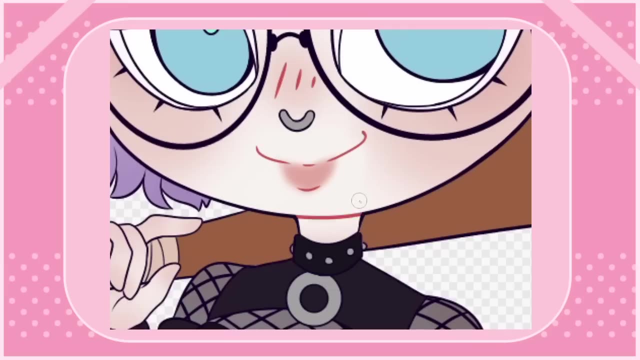 Trust me, I know this so well from lots of experience. It's not just as easy as get over it, but you can certainly take steps to stop comparing yourself or to hate your own work. Hey, improvement might be slowing and sometimes the pressure is real and being an artist is. 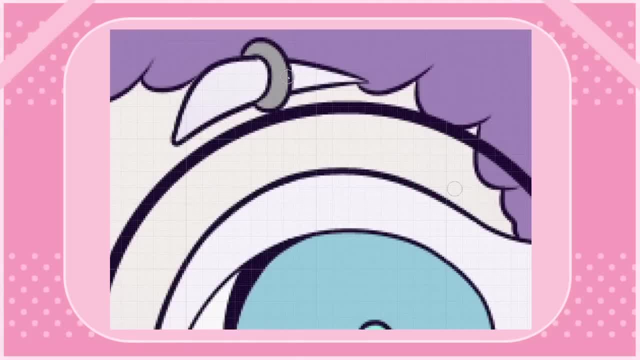 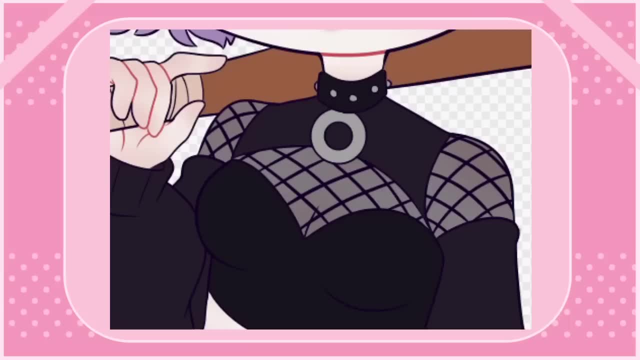 hard, but just keep going. Keep doing the things that you love. work on your passions. Don't focus too much energy on improving or measuring up to others or having a presence on social media. Just doing what you love will reap its own rewards. 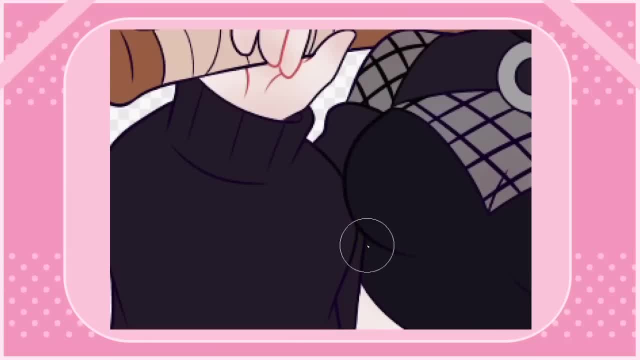 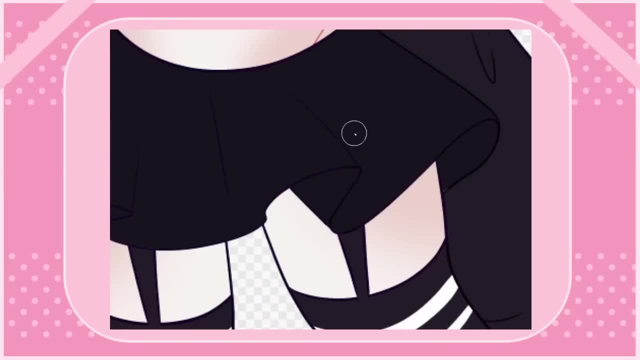 Also in line with doing what you love. another tip that I have is to draw for yourself and not for other people. I've known a lot of people who would draw things not because they wanted to, but because those things were popular, and I've actually done this before myself. 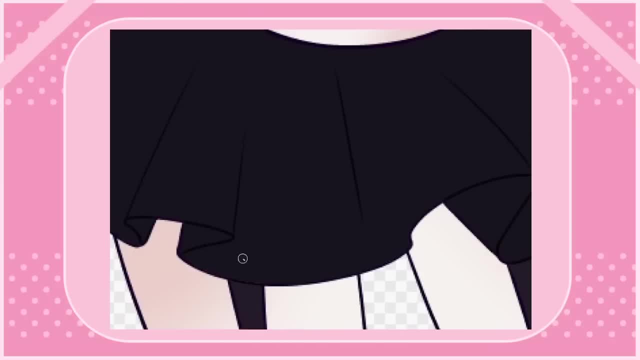 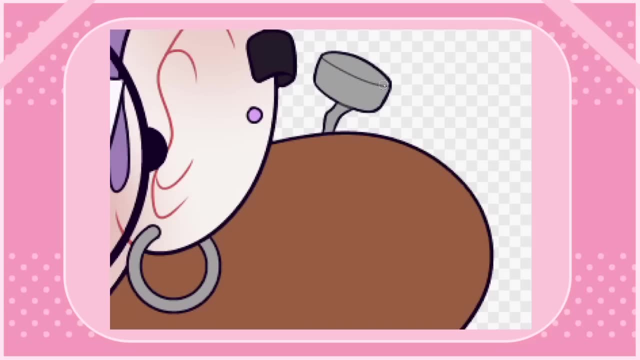 Forcing yourself to make art of things that you're not interested in is going to cause you a lot of grief in the long run, as art will be less fun and you may even grow to resent it. For example, I used to draw a lot of has-been hotel and hell of a boss art because people would respond to those works more than they would works on their own. So if you want to make art of things that you're not interested in, make art of things that you're not interested in, you can look into some of the works that you're. 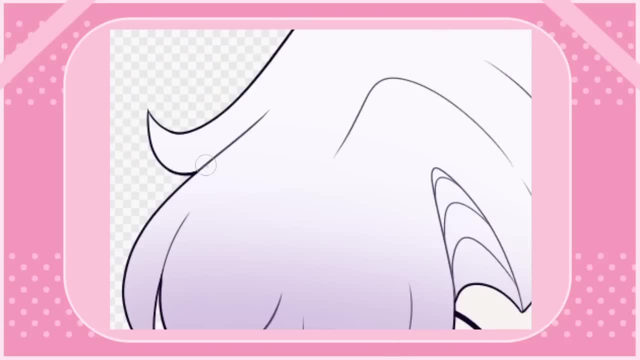 interested in drawing. I'd even draw more of them and then draw them against my own, or rather my own passions or OC's at the time. Of course, I didn't just start drawing them for no reason. I did like the show, but I definitely drew more of them just because they got more you. 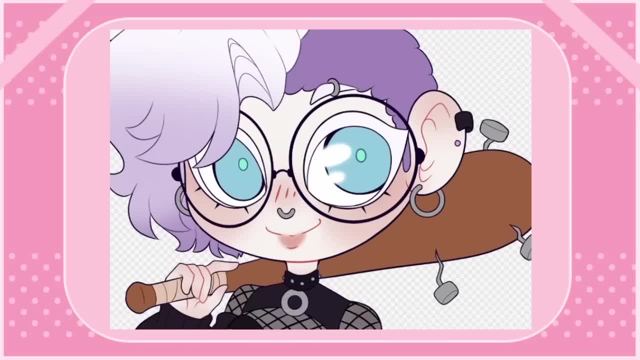 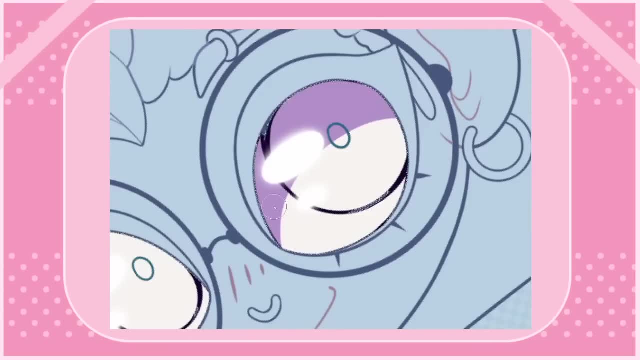 know sort of views and favourites on DeviantArt and stuff like that. In recent times I have actually come to slowly resent many of those works because they still get likes and favourites to this very day and it annoys me that some of my attention 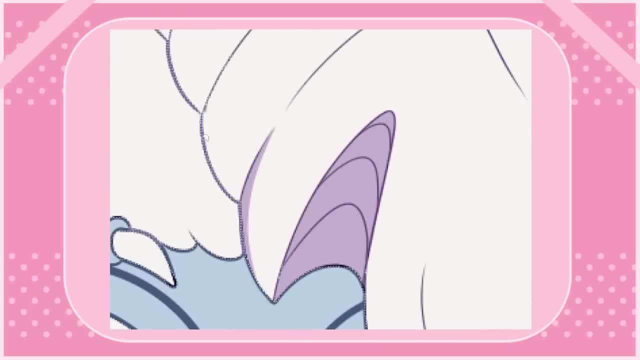 is not on my current like much better, much more passionate work. Drawing things that you don't want to draw for the sake of others is something that I just definitely advise you stay away from. That's what makes this work more fun and it's awesome. 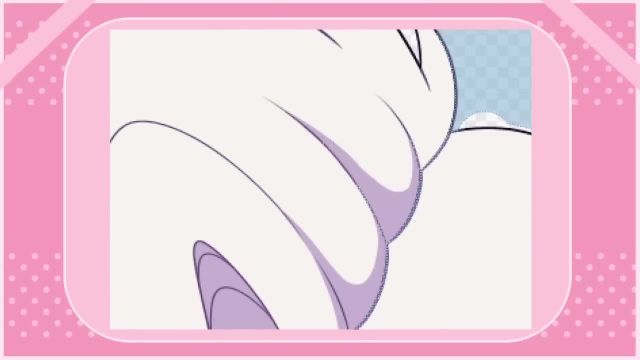 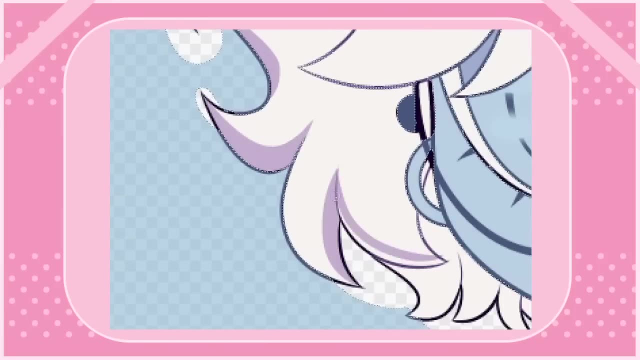 Finally, I want to talk about how to take criticism Now. growing up, I was exposed to a lot of commentators and DA-ranters that would bring up this whole criticism of quote. Person X doesn't take criticism, so they're bad. 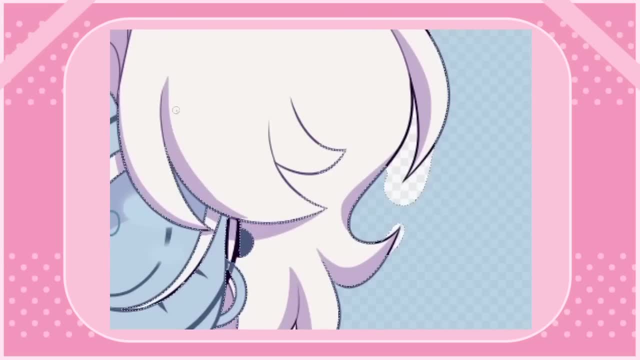 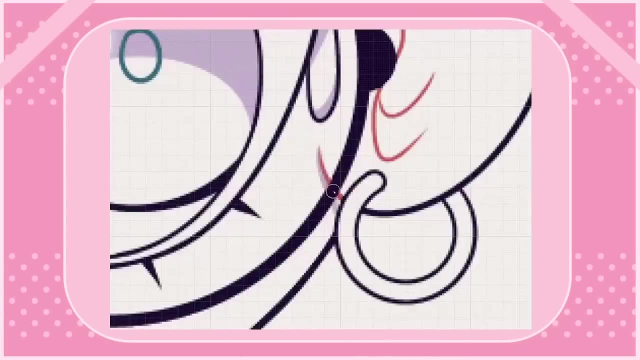 And, frankly, this sort of thing just kind of embedded itself into my mentally ill, neurodivergent brain and insisted that I have to take critique from each and every person who would give it and that I would be obligated to ask for critique even when I would be in a state where 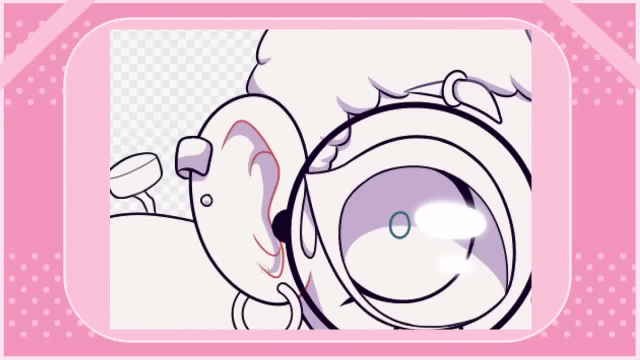 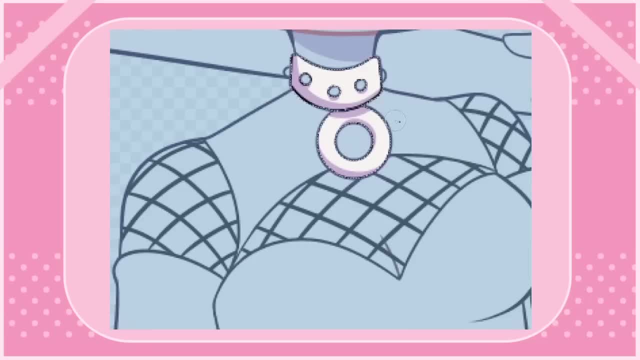 I couldn't handle it or didn't want it. So, yeah, I want to sit down here, pop a squat and tell all of you that all of that stuff that I believed and many other people pushed is a total, ripe crock of shit. 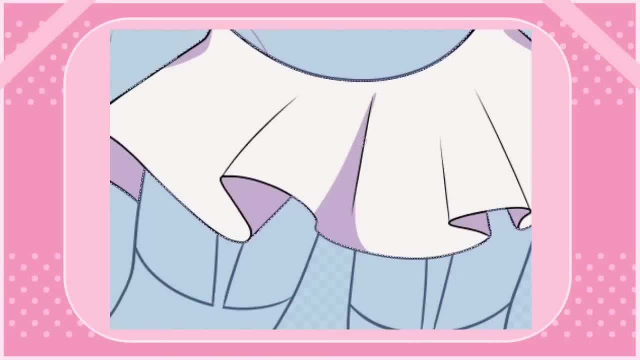 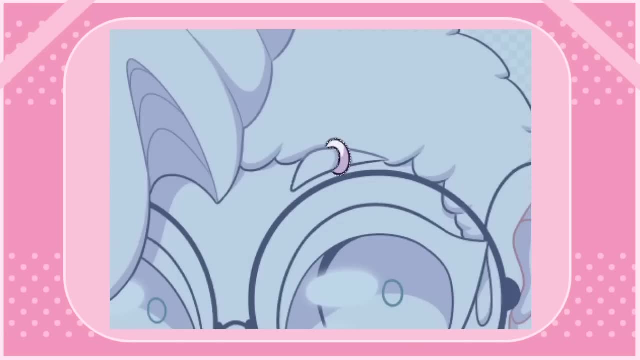 Someone's art and personal passions are a very sensitive subject, and it's not wrong for them to state that they do not want or are not open to criticism of their work. So yeah, if you're an artist like me who tends to be sensitive about criticism, then 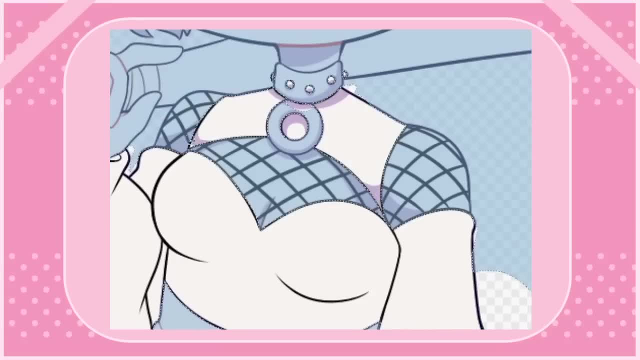 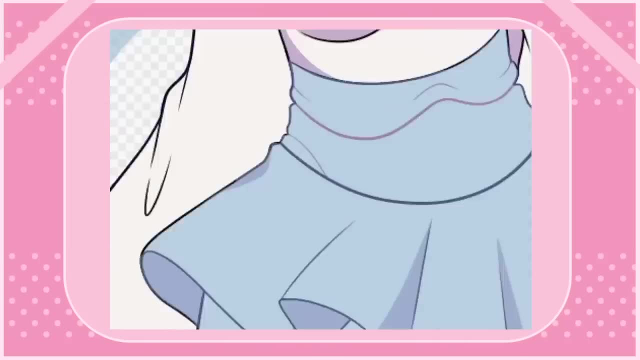 you're not obligated to take it nor to open yourself up to it. This is especially the case when the critic berates you or is completely destructive, Or when they offer worthless criticism like this is cringe, or this is ugly, or this looks. 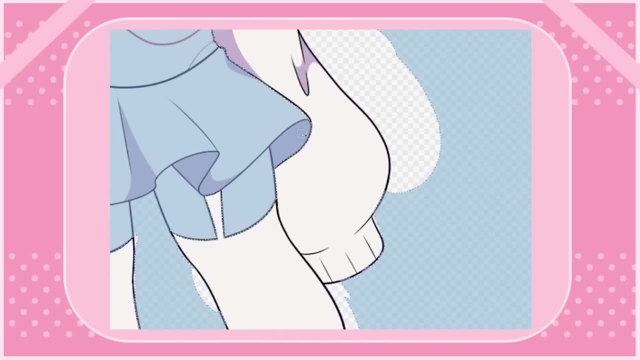 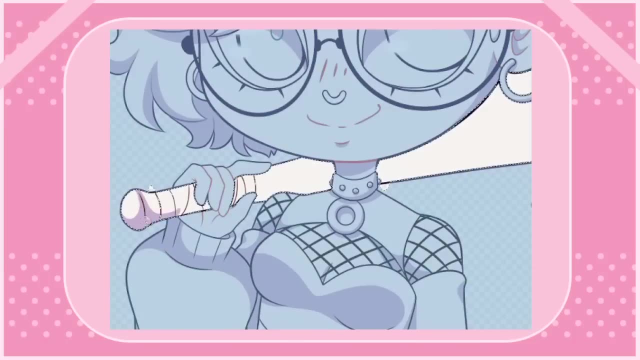 weird. All of those things are not helpful and don't really give the artist any clear ideas on how to improve. Now, on the other side of that coin, though, I want to say that I recommend being at least open to critique. Of course, no one is obligated to take critique or to be open to it, but if you're looking 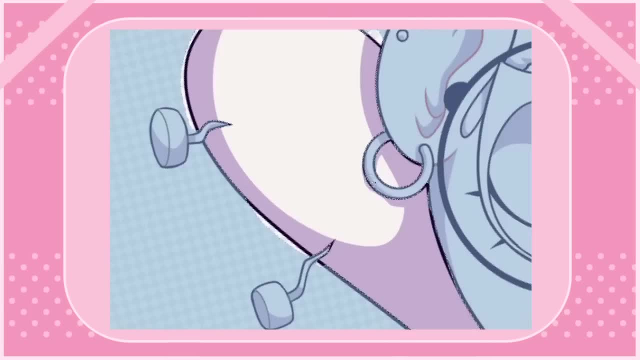 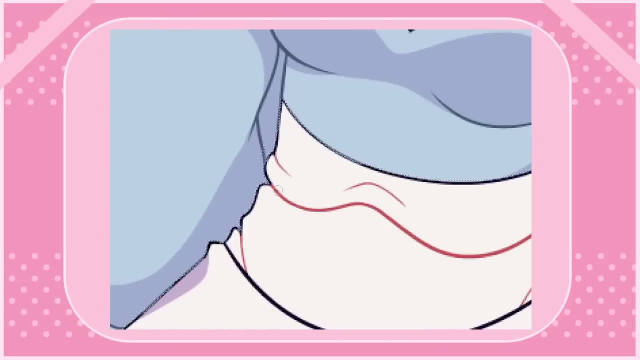 to improve, then it's good to search for constructive critique from someone who you can tell is in good faith. When someone says, hey, I noticed that the leg here is a bit too short, Then perhaps taking that criticism, evaluating it and then, if it's valid, implementing. 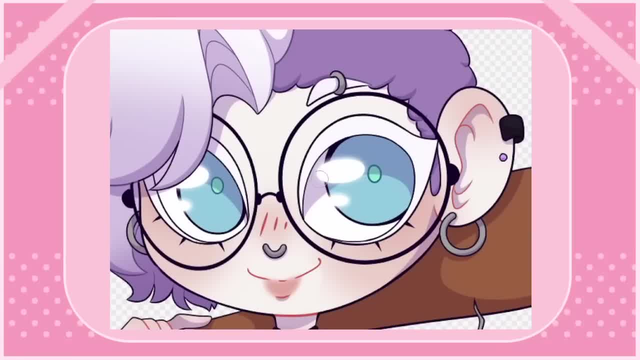 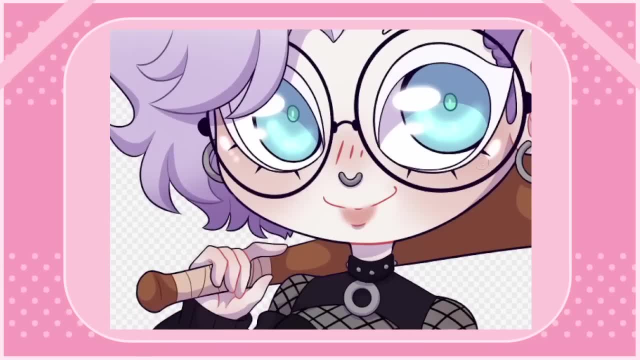 it will actually help you improve your work. The whole taking criticism thing is admittedly a bit of a balancing act. I think that it's best to be open to constructive critique but to not feel pressured to take criticism that is confusing, destructive or invalid. 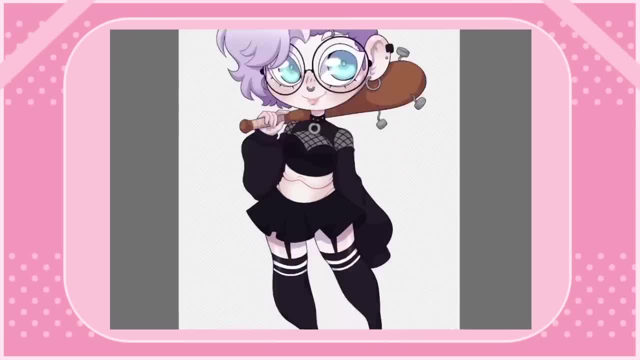 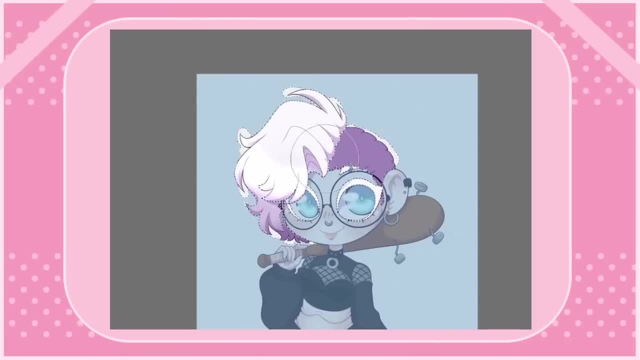 Please be open to suggestions, but, just like requests and commissions, you don't have to do something that someone suggests that you don't think is valid. Furthermore, you don't even have to acknowledge criticism if you decide to take it. If someone says the leg is too short, you can make sure to fix that in future pieces. 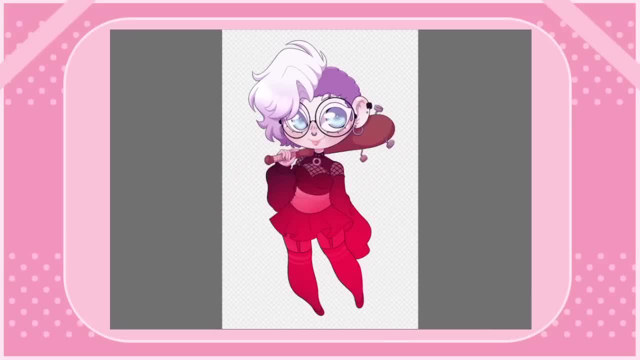 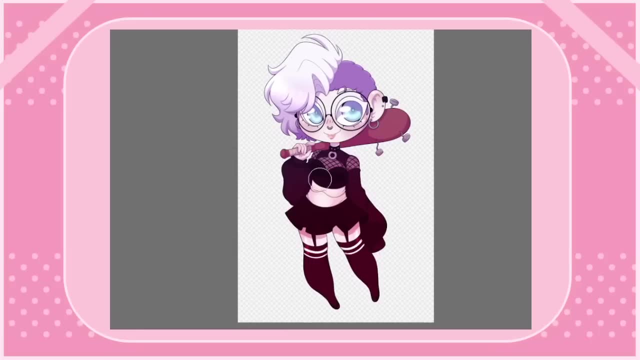 but you don't have to give the person who gave the critique validation, especially if the criticism was delivered or presented in a rude or abrasive fashion. Anyway, that's all I really wanted to say for this video. If you'd like to add your own additions to my art tips in the comments, then I would. 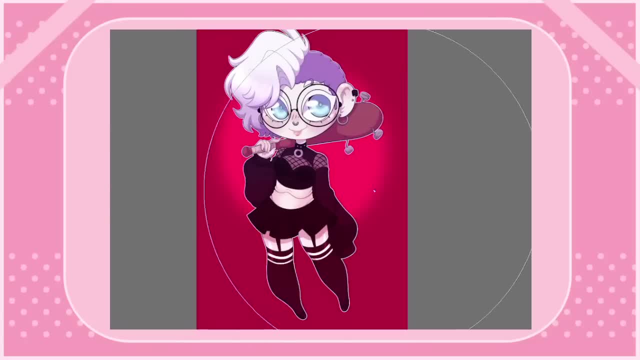 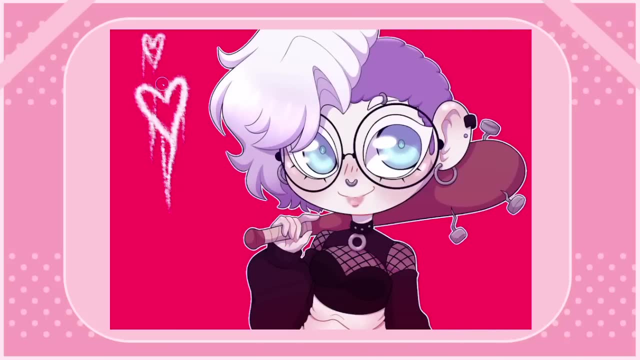 love to hear some of your suggestions and ideas and experiences. If you're a beginner artist, struggling or just a little bit less experienced than I am, I hope that some of these tips and suggestions were helpful to you. With all of that being said, 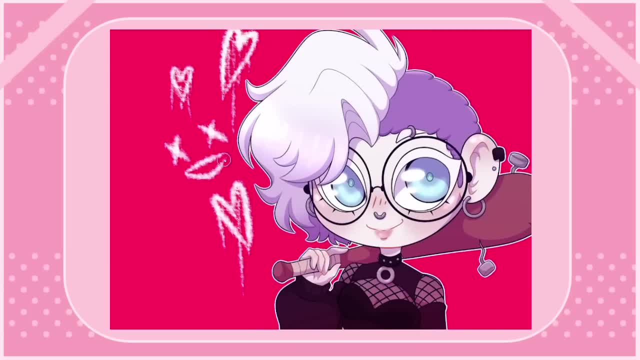 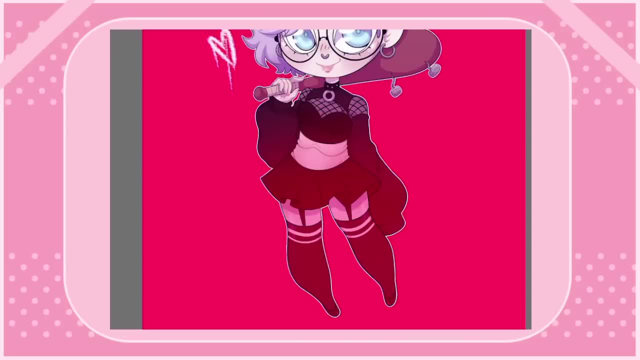 I hope you enjoyed this video. If you liked it, feel free to rate and subscribe if you'd feel inclined to do so. If you want to see some of my art and writing safe for work and not safe for work- 18 plus for that last one- or if you just want to see some of my crackhead tweets, then follow. 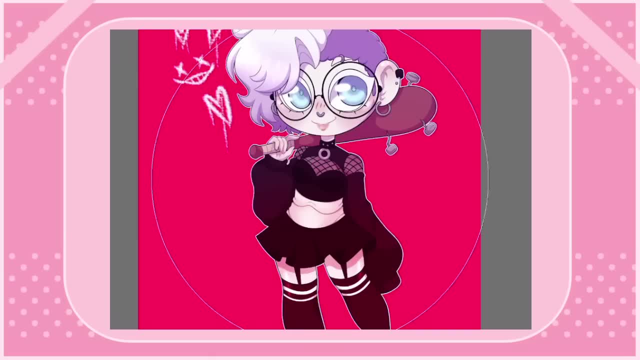 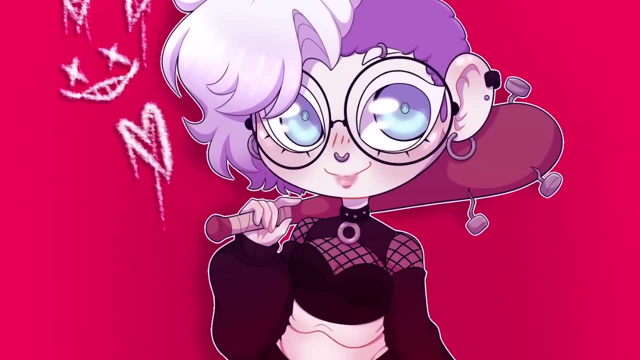 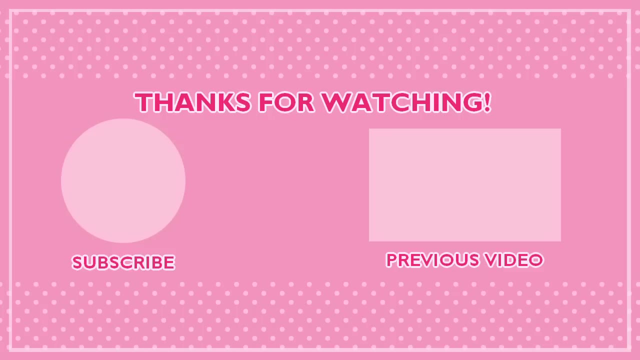 the link to the card in the description, where you can find the links to all of my social media. Thank you for watching. I hope you have a nice rest of your day and don't forget to stay magical. Bye, Bye, Bye, Bye.